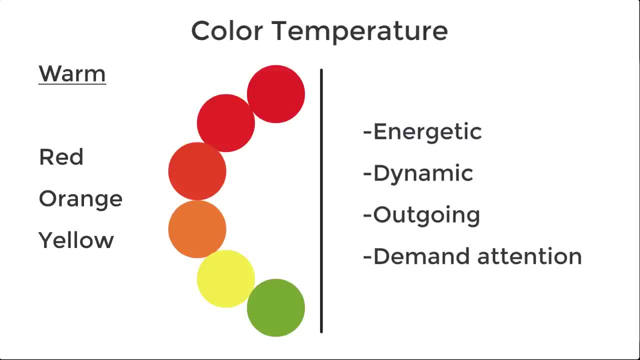 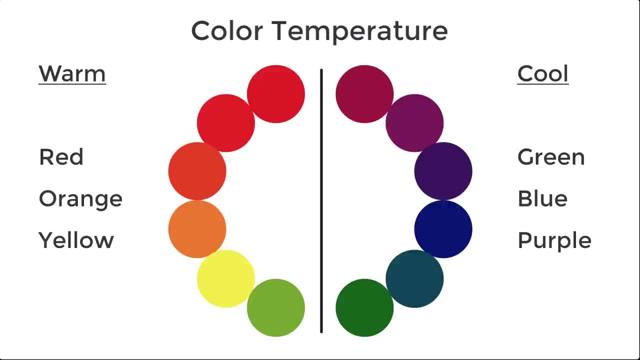 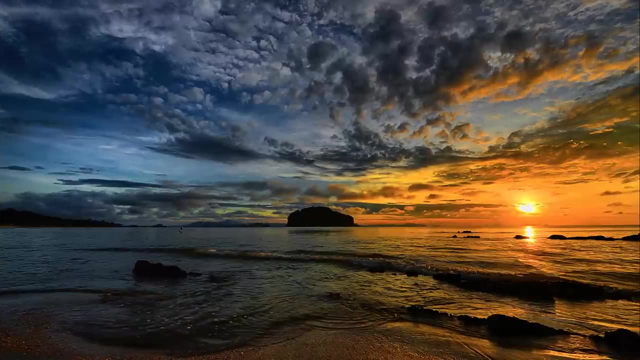 purple. Warm colors are perceived as energetic, dynamic, outgoing, and they demand our attention more than cool colors. Cool colors are generally perceived as distant, restrained and calm. Warm colors are said to advance to the eye, while cool colors recede to the background. 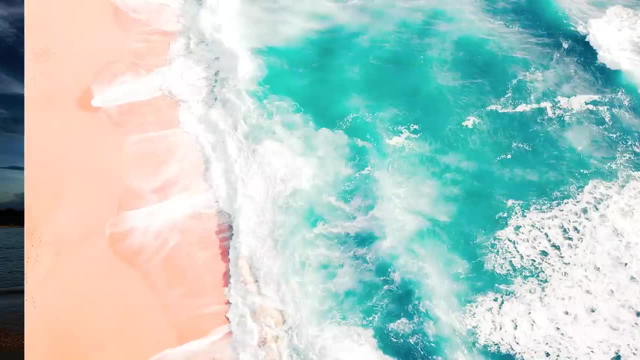 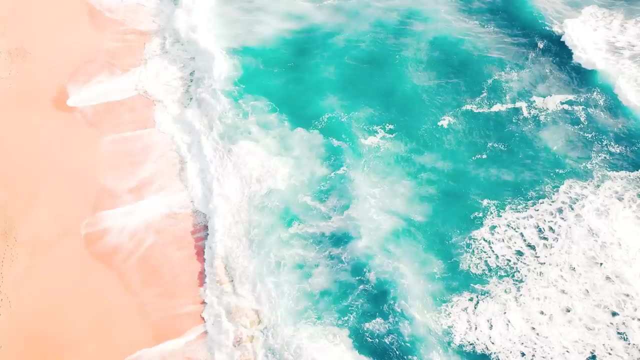 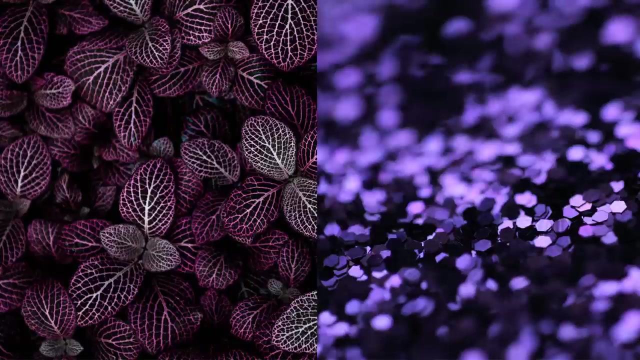 However, there are exceptions to this rule. A vivid, pure, cool color will appear to advance and overwhelm a subtle, grayed, warm color. You can also alter the temperature of a color by changing its undertone. A cool color with warm undertones will take on more of that color's characteristics and 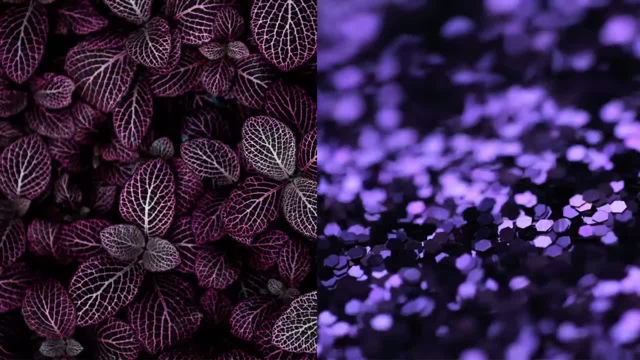 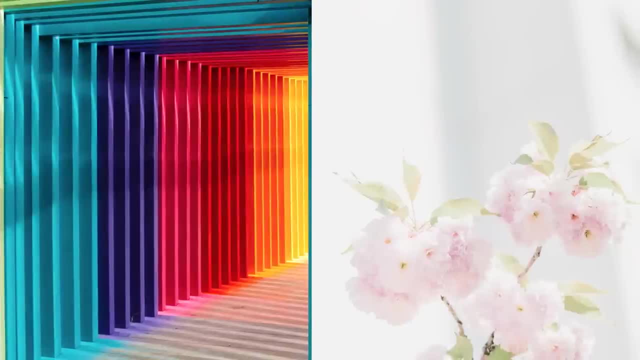 vice versa. For example, a reddish purple will be perceived as a warm color. It will be perceived as warmer than a cool bluish purple. The saturation and value of a color can also have a big impact on the way we perceive that. 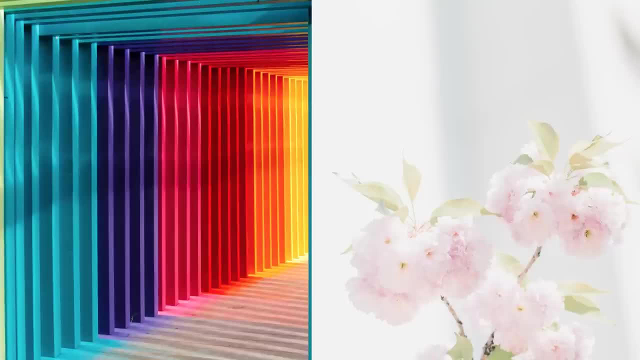 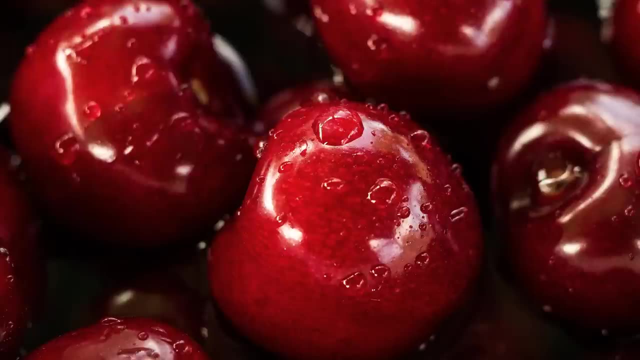 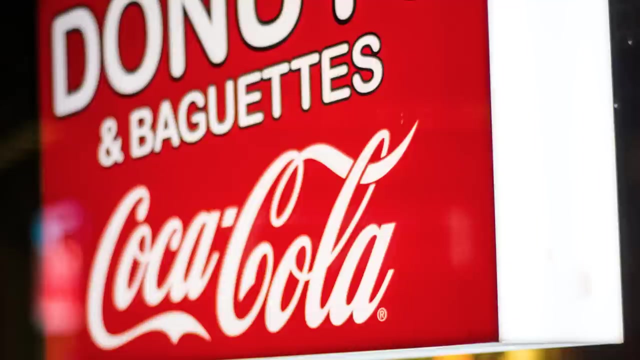 color psychologically. Now let's take a look at the significance of each color, beginning with red. Red is a color that we, as humans, react to very strongly, both psychologically and physiologically. Red can excite, alert or engage us. 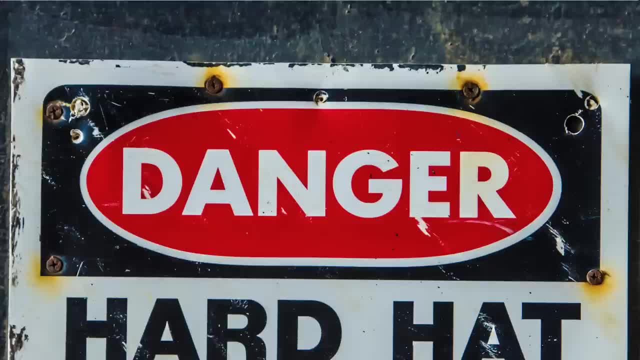 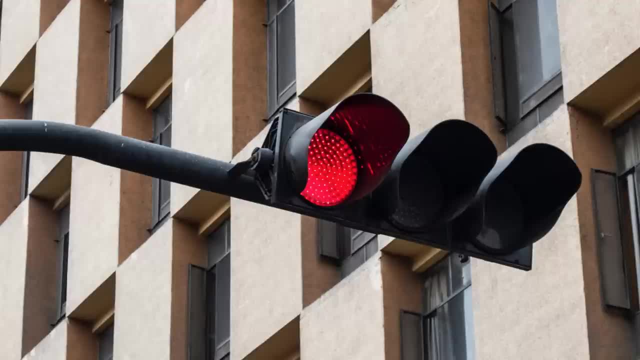 Red is known to increase our appetite. Red is known to increase our heart rate, pulse rate, muscle strength and blood pressure. It also causes an adrenaline rush. We notice red above all other colors and we are hardwired to act or react to it. 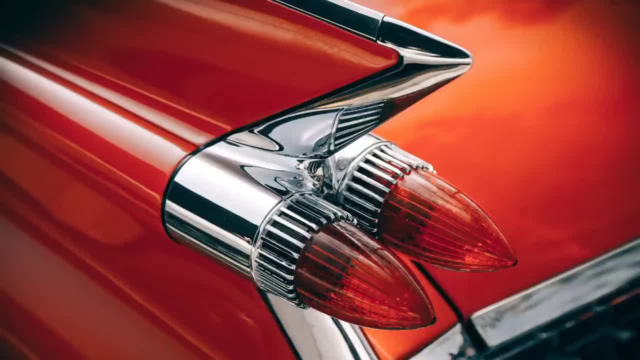 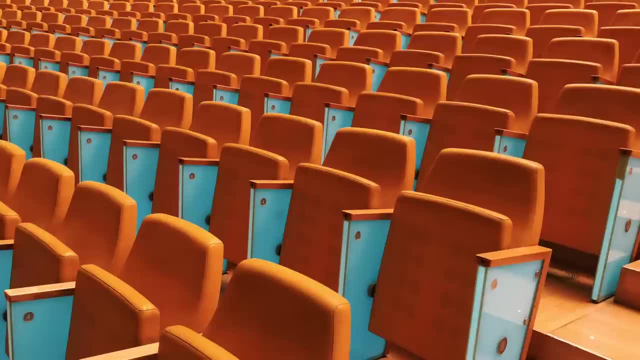 We generally perceive red as intense, passionate, powerful and exciting. It is a color of love, danger, anger and sensuality. Orange is known to encourage social interaction. It makes us feel content. It boosts oxygen supply to the brain. 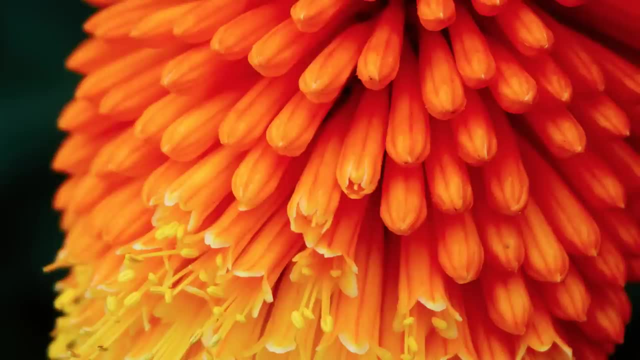 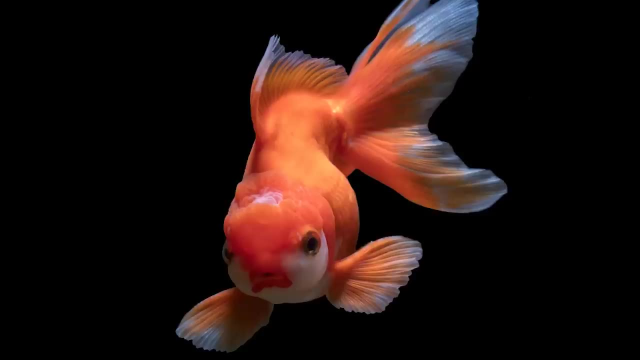 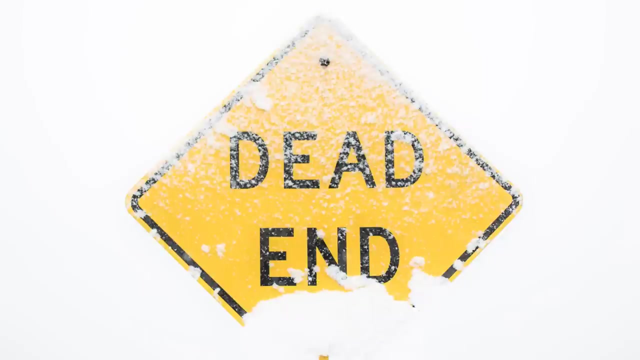 Red is known to increase our appetite. It causes our attention. We generally perceive orange as friendly, warm, playful and energetic. It is the color of creativity, wisdom, happiness and friendship. Yellow is known to trigger spontaneous action and it can make us feel hungry, perhaps because 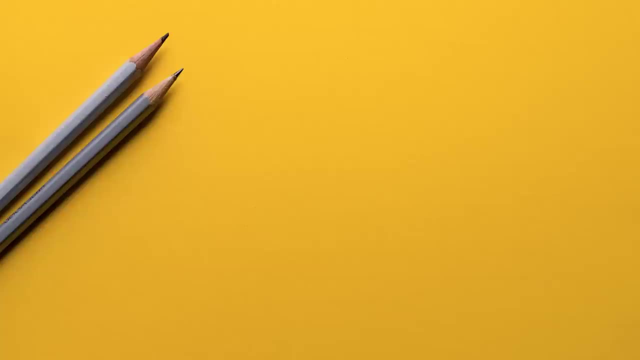 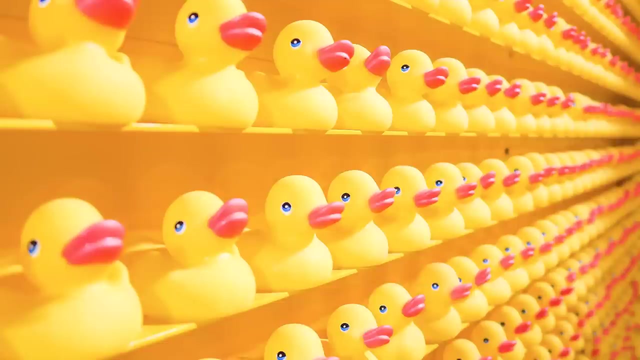 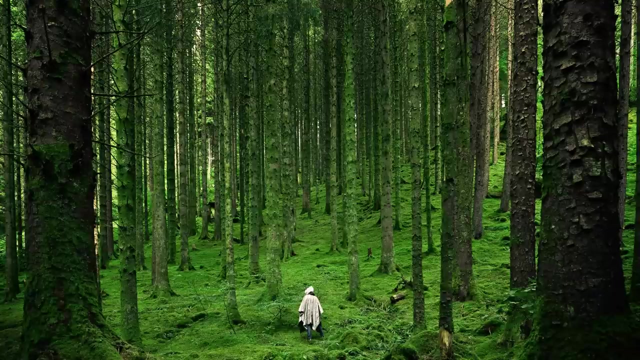 it reminds us of comfort foods like mac and cheese, french fries and mashed potatoes. We generally perceive yellow as bright, positive, joyful and fun. Red is known to increase our appetite. It makes us feel content. It is the color of joy, hope, enlightenment and sunshine. 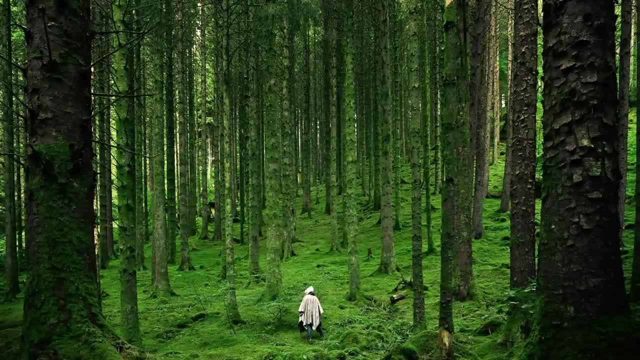 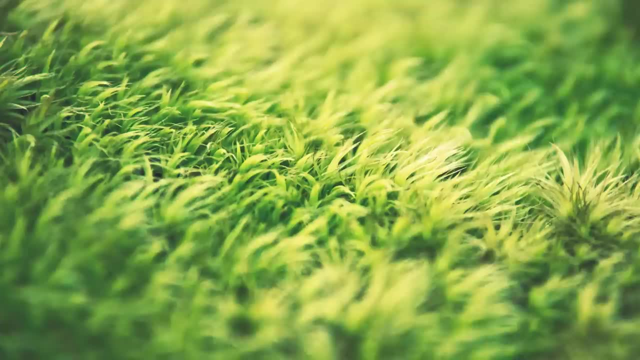 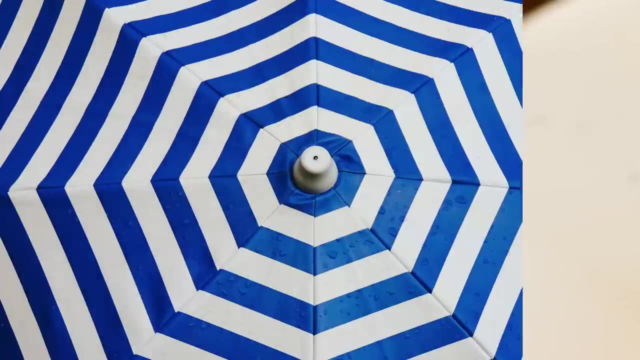 Green is known to make us feel calm and safe. It promotes freshness, inner peace and tranquility. We generally perceive green as peaceful, youthful, harmonious and relaxing. It is the color of nature, balance, harmony and fertility. 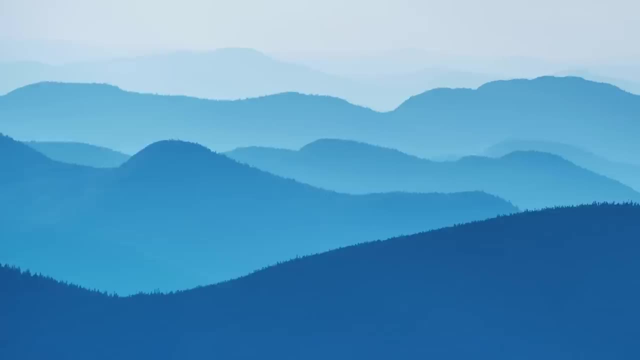 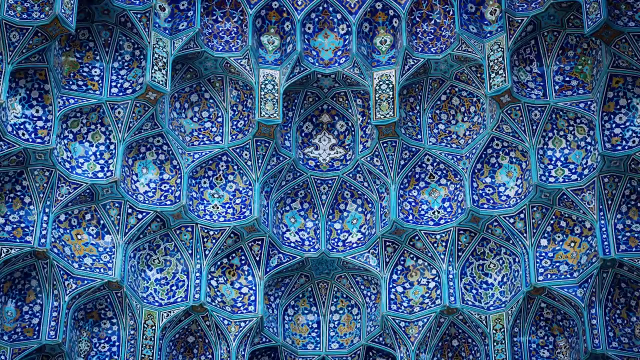 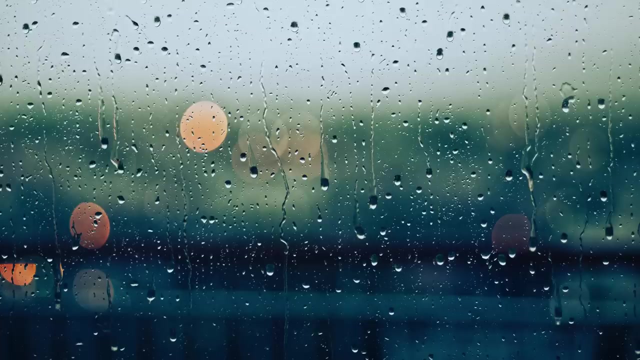 Blue is known as a dependable and soothing color. It is extremely popular with young people. It is extremely popular and widely used in all types of branding. We generally perceive blue as serene, inspiring, trustworthy and innovative. It is also sometimes perceived as gloomy, sad and melancholic. 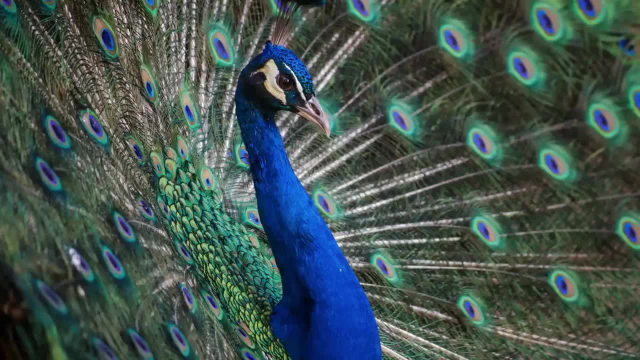 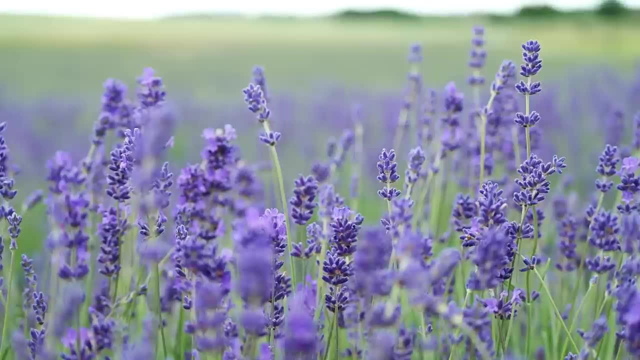 It is the color of freshness, freedom, sincerity and authority. Purple is known as a mysterious and elegant color. Purple dye used to be so expensive and difficult to make. It is the color of freshness, freedom, sincerity and authority. It is the color of freshness, freedom, sincerity and authority. 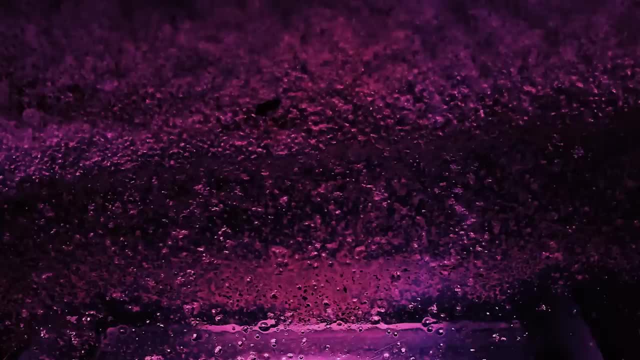 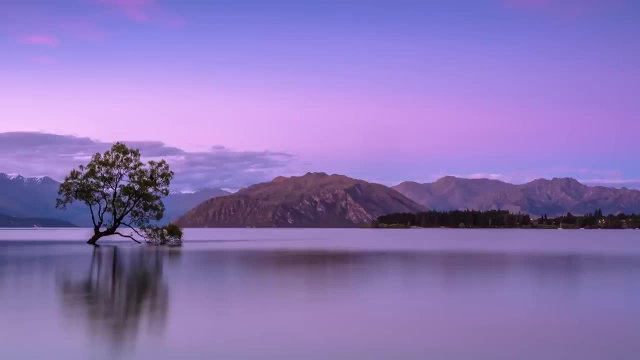 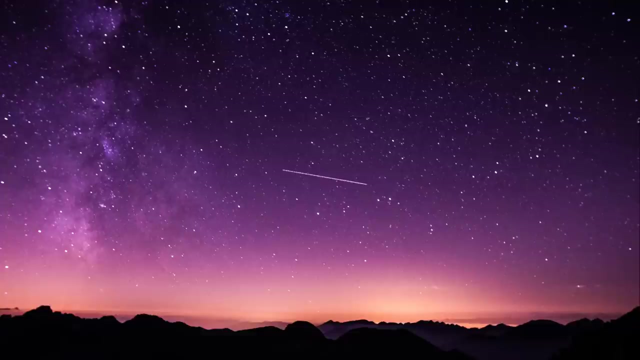 Only royalty or the extremely wealthy could afford it. This is how it became known as a royal color. We generally perceive purple as spiritual, dignified, magical and majestic. It is the color of imagination, mysticism, intuition and integrity. 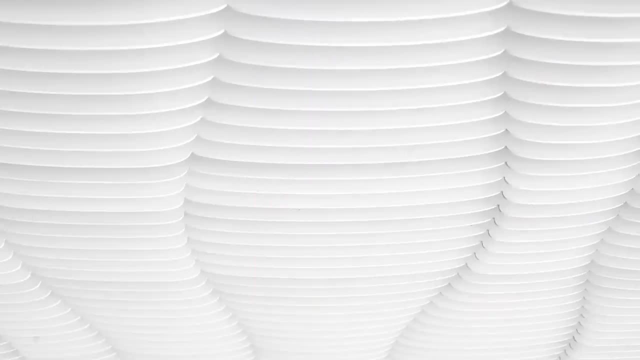 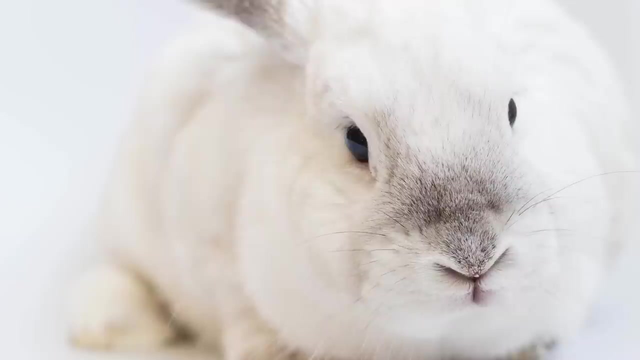 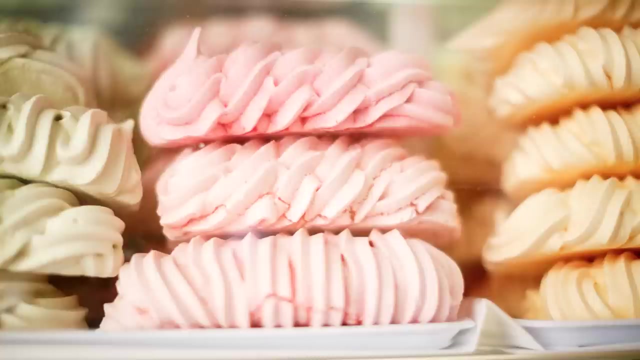 It is the color of pure, clean, calm and light. We generally perceive white as pure, clean, calm and light. minimalism In color mixing- adding white to a color will make it lighter, softer and understated. Pastel colors are created by adding large amounts of white Pastel colors. 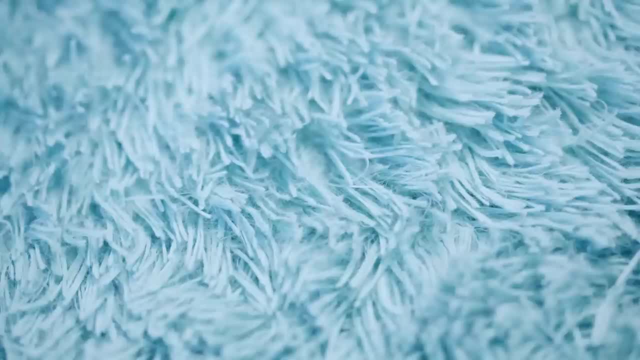 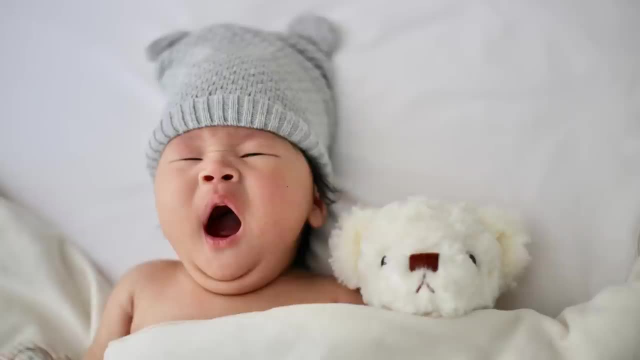 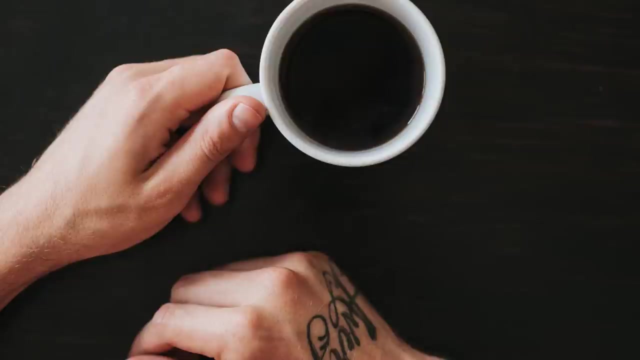 are generally perceived as sweet, gentle, intimate and childlike. They are the colors of candy, babies and innocence. Black is known to have an imposing, solid, serious and permanent presence. We generally perceive black as dark, cynical, modern, sleek and 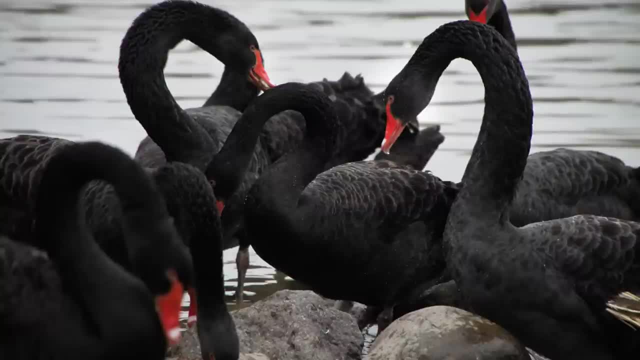 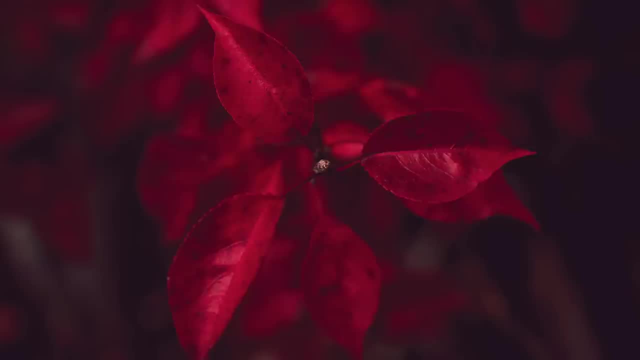 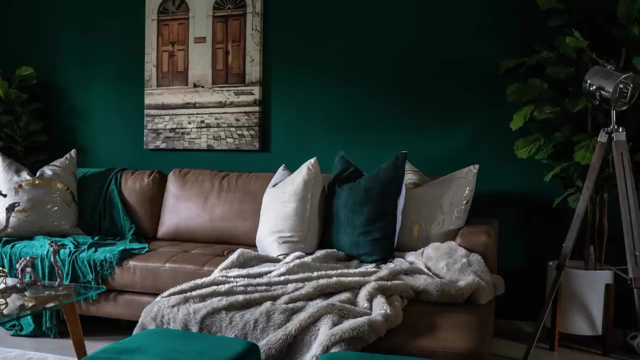 confident. It is a color of deceit, elegance, piety, mystery and sophistication In color mixing. black can be added to a color to make it darker, bolder or deeper. We generally perceive deep, dark colors as luxurious, regal, indulgent or sinister.